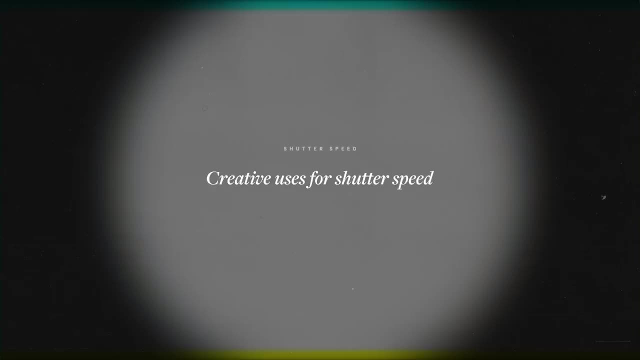 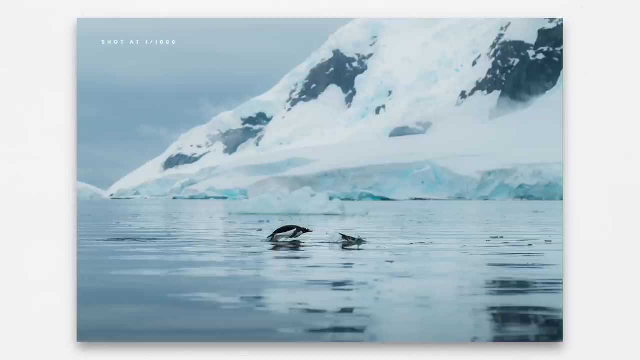 able to make its way onto the sensor Now creatively. the way to think about shutter speed is to think about whether or not you want to freeze the action in your image, or whether you want your image to be blurry, To freeze the action, which is going to be most of the time, especially if you're shooting. 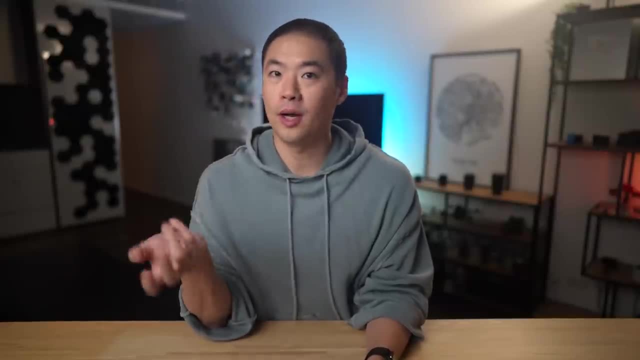 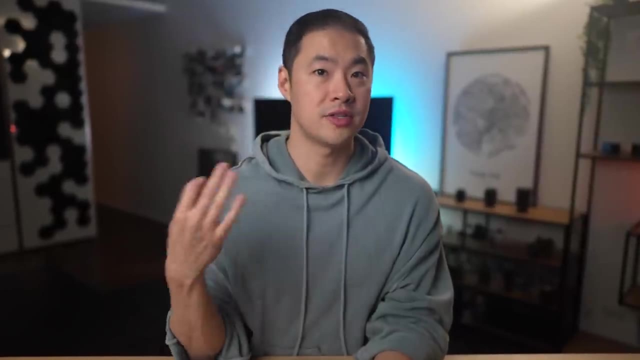 you know street or portraits or sport or wildlife, etc. you want a faster shutter speed typically. so you know 1 over 250,, 1 over 400,, 1 over 800,, 1 over 1600 and so on When it comes to freezing. 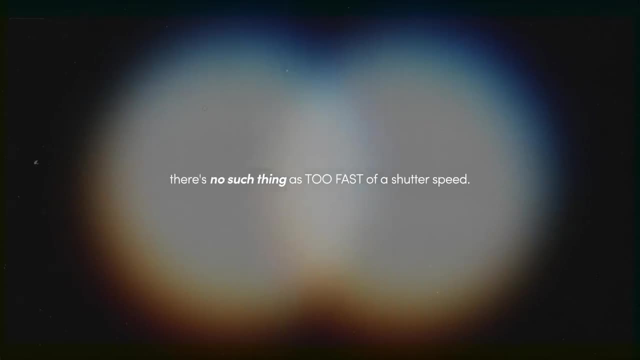 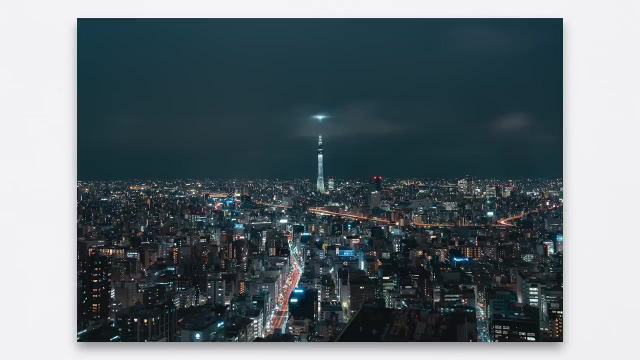 the action. there's no such thing as too fast of a shutter speed. Now, if you have a tripod to rest your camera on, then you might be doing night photography or landscapes and you might use slower shutter speeds, such as one second, two seconds, four seconds, eight seconds or more. 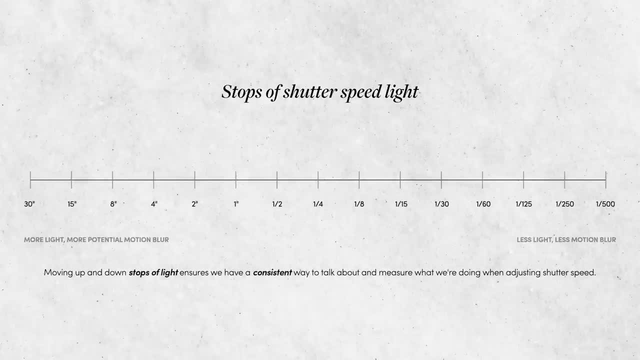 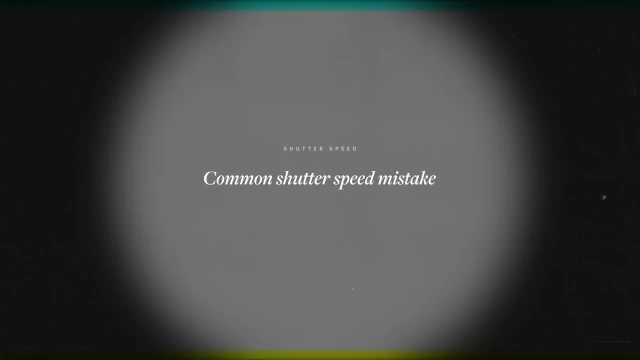 Now, all of these denominations are actually one step of light difference between each other and for shutter speed. this is how we talk about it in time. One common mistake that people make when they first start out with photography is that they complain that their images just aren't sharp. 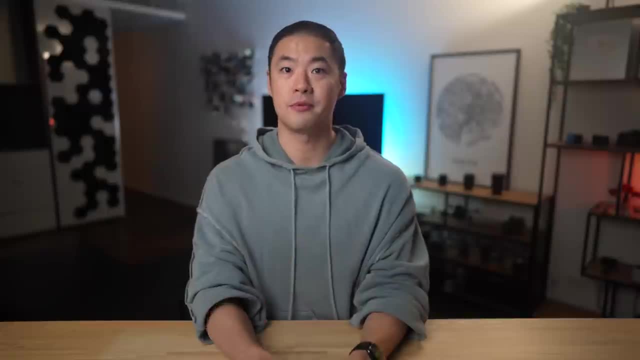 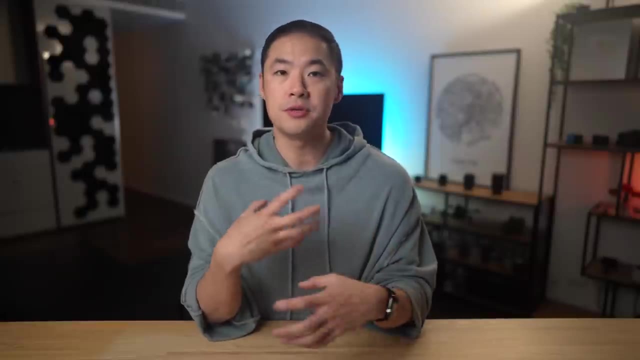 that isn't because they don't have good gear- you know, most cameras are actually pretty good nowadays- but actually it's because they don't have a fast enough shutter speed and they're introducing micro rigidist and therefore blur into their images. Check out this video I made. 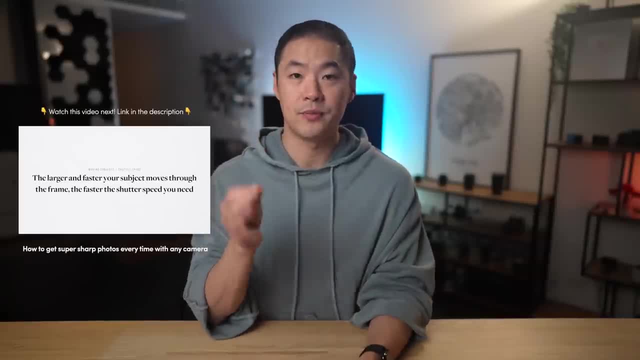 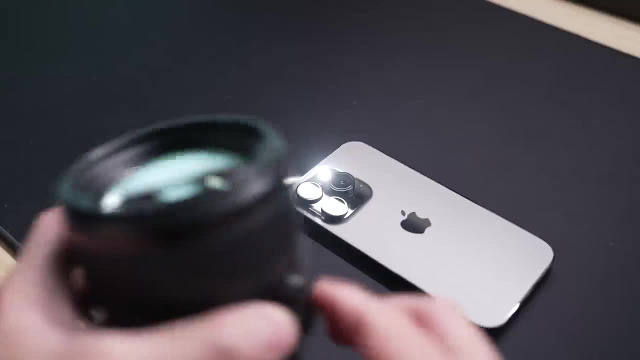 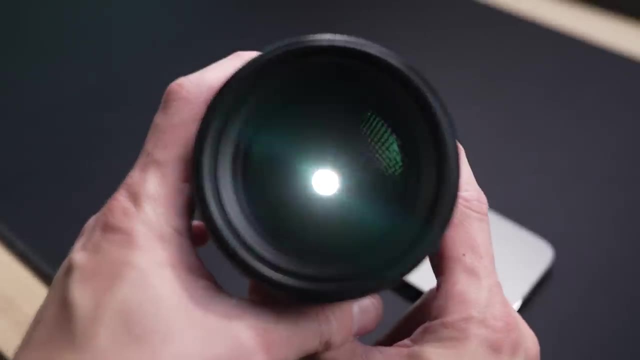 here if you want to ensure that your images are absolutely tack sharp every single time. The second component of the exposure triangle is called aperture. The aperture refers to the size of the opening at the end of the lens. The more light comes through, the smaller the iris, the less light comes through. 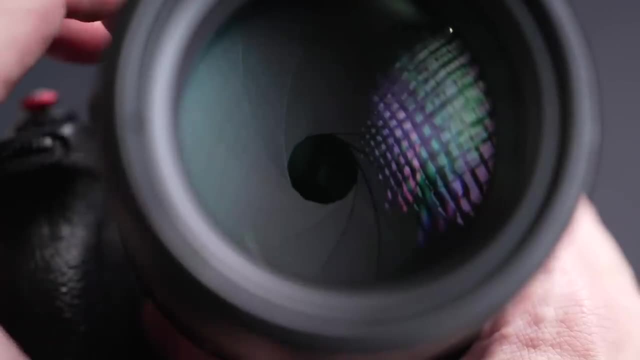 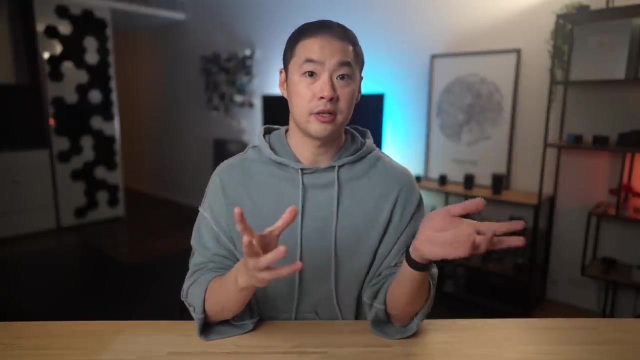 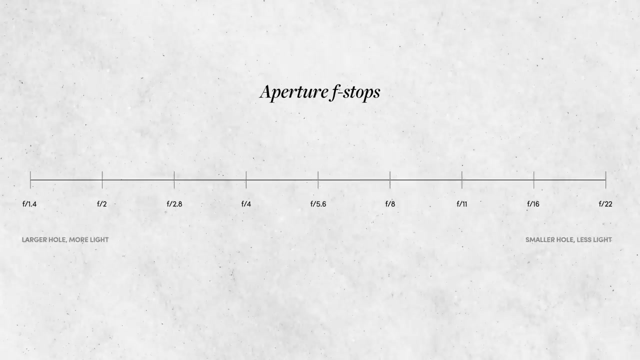 For aperture. we refer to stops of light that it produces as what's called f-stops. The closer to zero that number, the larger the aperture will be. the larger the number, the smaller the aperture will be. So common aperture stops look like f1.4, f2, f2.8, f4, f5.6, f8, f11, f16 and so on. 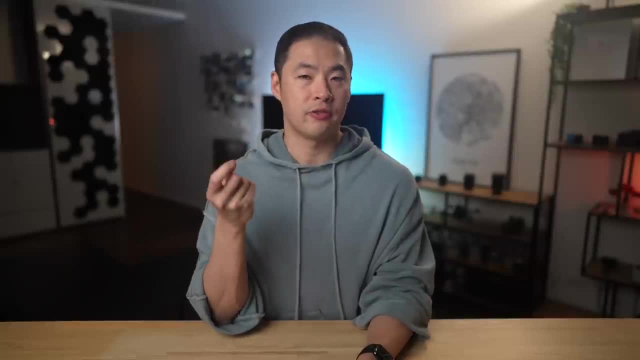 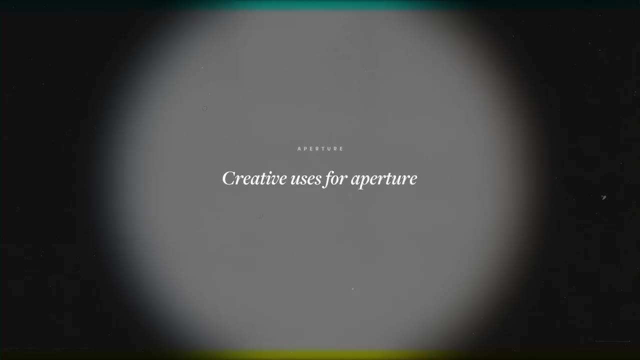 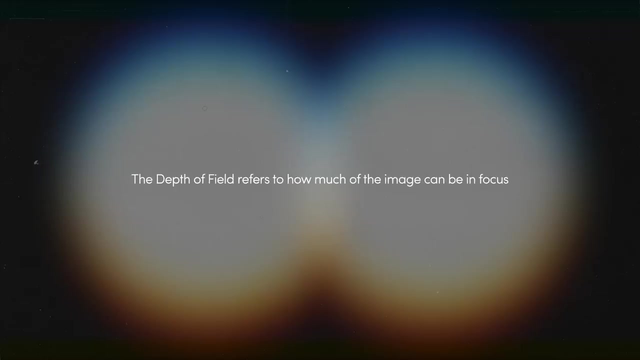 And, for example, lenses that have a maximum aperture of f1.4 will have a very large aperture like this one, Now, creatively. aperture is most commonly associated with controlling what's called the depth of field. Simply put, depth of field refers to how much of the image can be in focus. 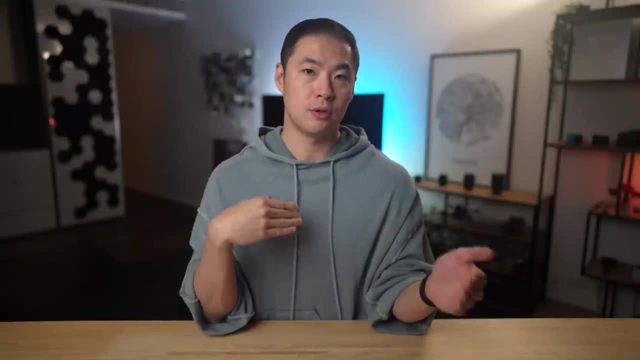 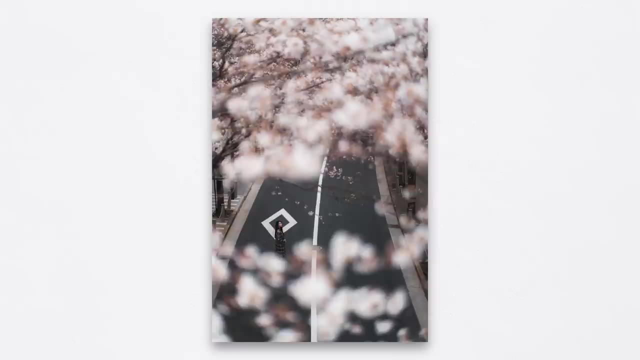 So large apertures like f1.4 will produce what's called a very shallow depth of field. This means that the area of focus is quite thin or is quite shallow, and it's typically used to draw your eye into the thing that's the most important thing in the composition, while the rest of the 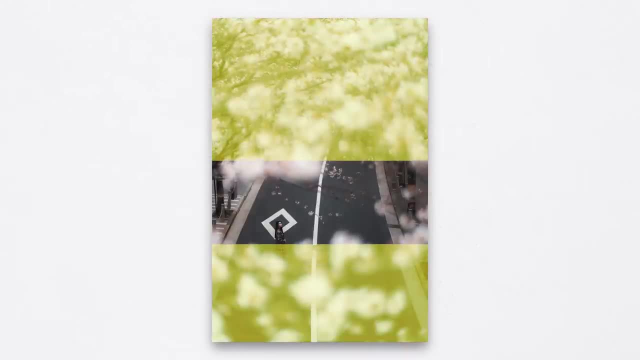 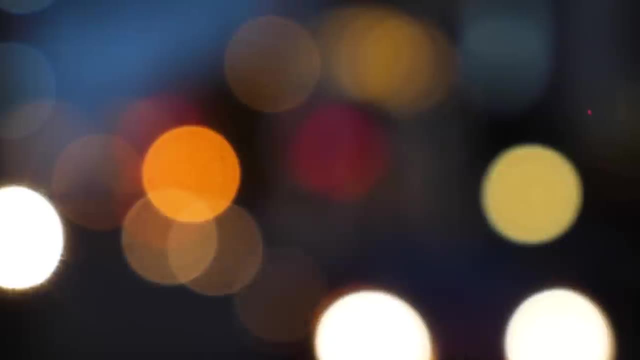 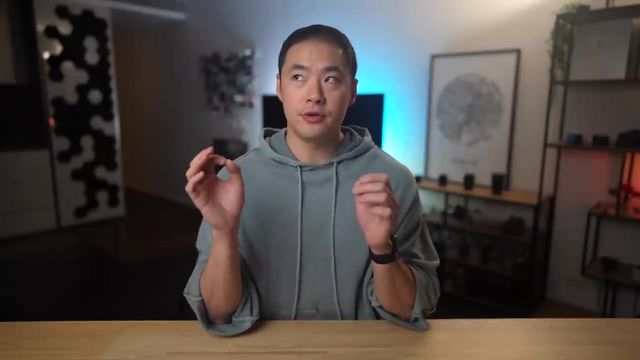 image goes out of focus, And this out of focus blur is commonly known as bokeh, and many people find it to be very aesthetically pleasing. These effects are very often found in genres such as portrait or fashion photography. Now, on the opposite end, if you do landscapes or architecture, 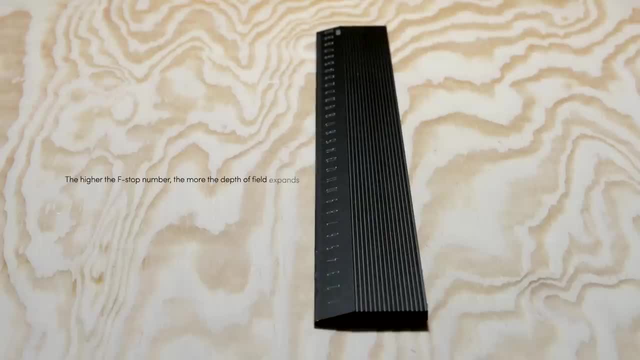 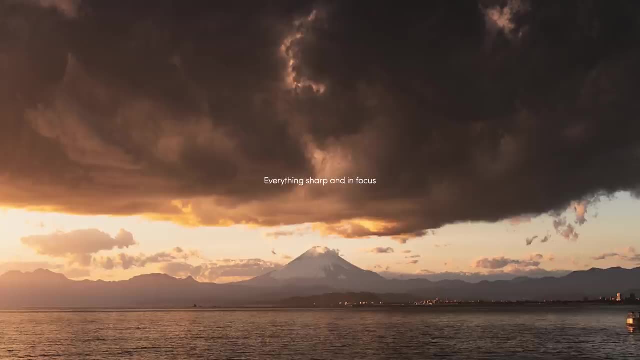 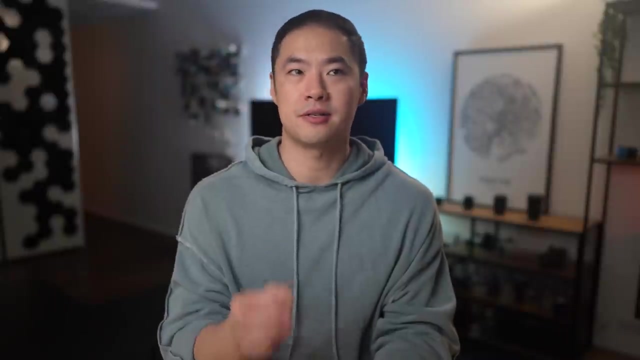 for example, you'll probably want a much deeper depth of field, So you would use a smaller aperture, such as f5.6, f8, f11, so that you can get everything in focus. Now, depth of field can get really, really detailed and complicated because it has many, many other factors, such as 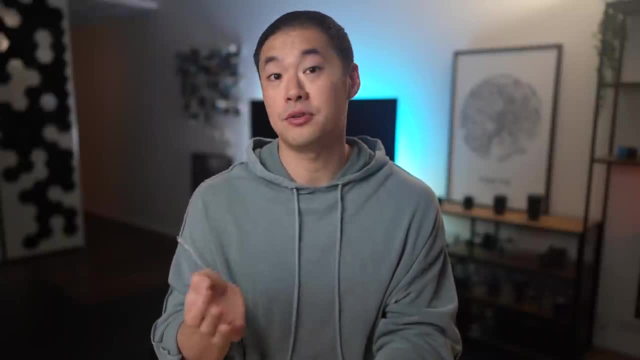 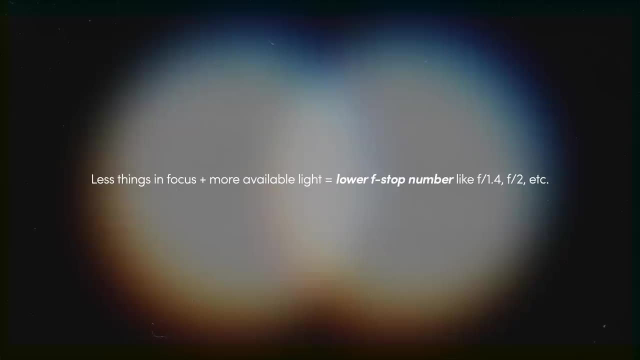 subject: distance, focal length and so on, but this is definitely enough to get you started. Just remember, if you want less things in focus but more available light, then a lower f-stop number like f1.4 will do the trick. If you want more things in focus but less available light. 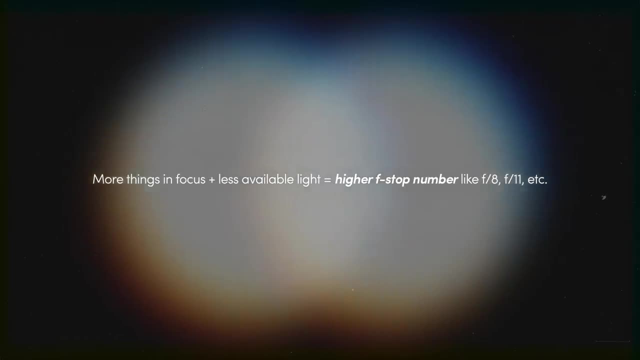 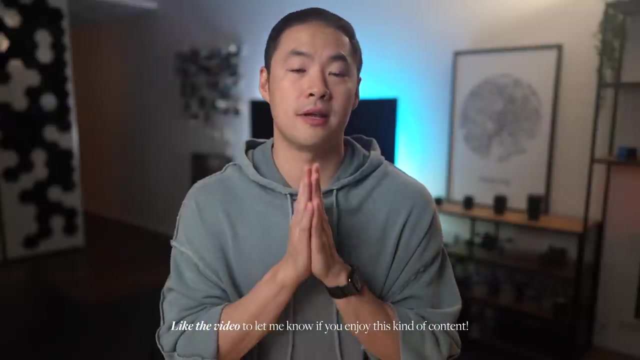 then a higher f-stop number, like f11, will do the trick. Okay, if you're enjoying this video so far, I would really appreciate it if you would hit that like button for me so that I know it's good enough to make even more free videos like this in the future. And the last component of the exposure. 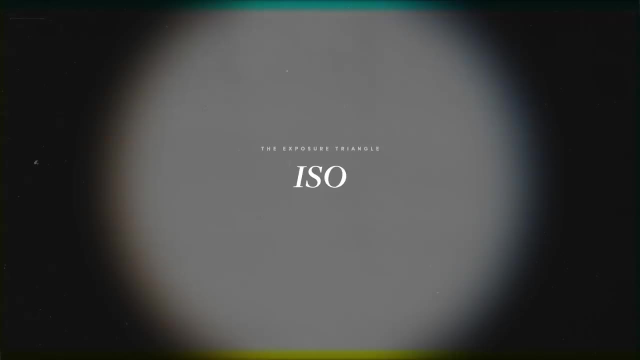 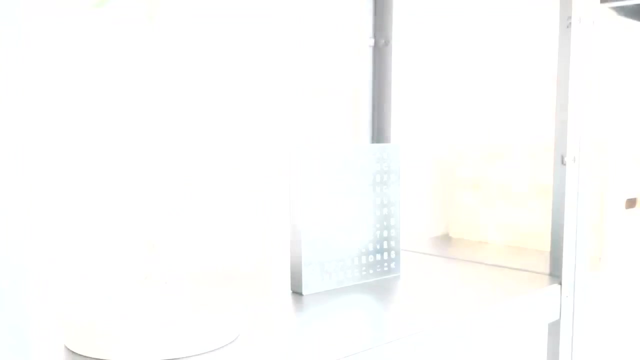 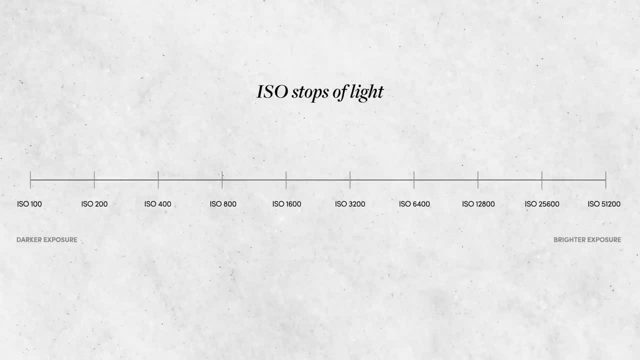 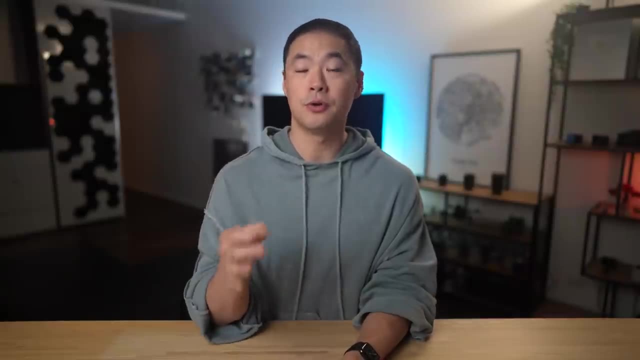 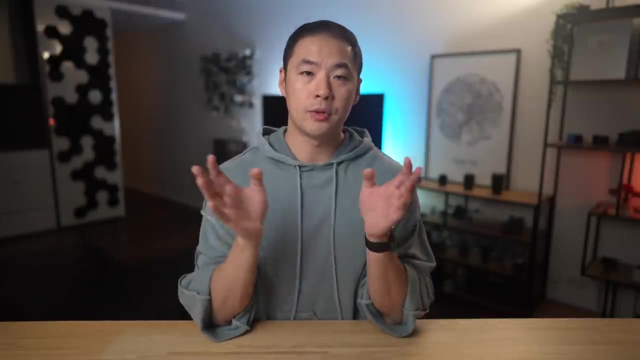 1600,, 30,, 200, 6400 and so on. Now, ISO doesn't have an implicit creative effect on our images like shutter speed or aperture have, and so it should also be treated in that way With ISO. the more you increase it, the brighter your image becomes, but also the more noise or visual 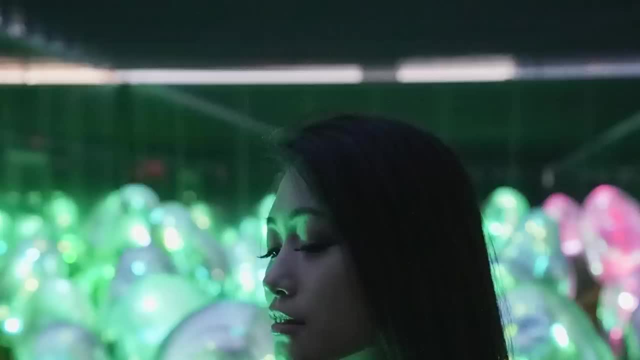 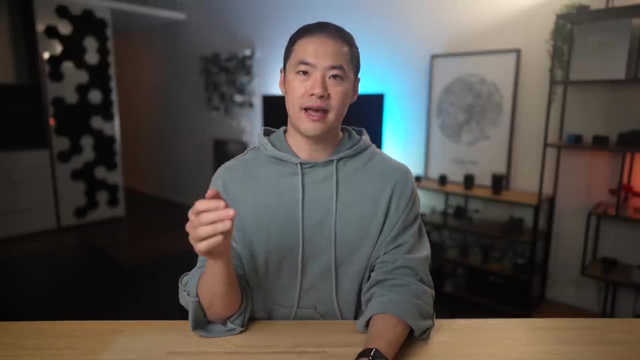 artifacts you introduce as well. You also end up decreasing dynamic range and color as well, but that's a very advanced topic for perhaps another time. Ideally, you want to have a as low of an ISO setting as possible, so long as your other two settings are correct. 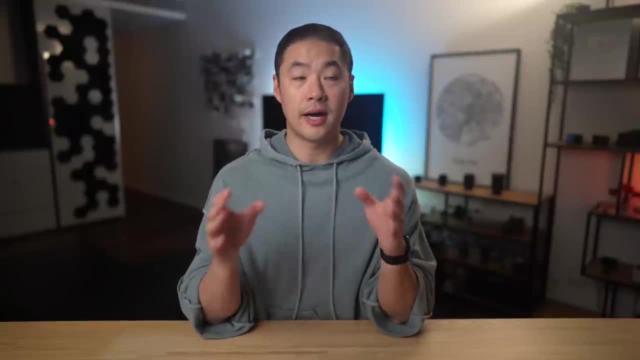 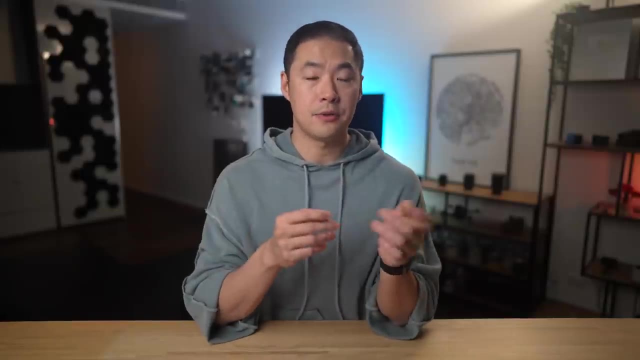 first, One very common mistake that beginners make is that they think ISO and noise is a huge, huge deal, so they keep it really, really low at the sake of getting their shutter speed or their aperture incorrect, and this is a mistake, You know: messing up your shutter speed or your aperture. 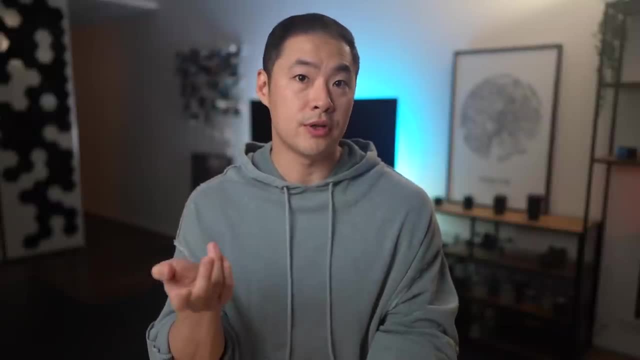 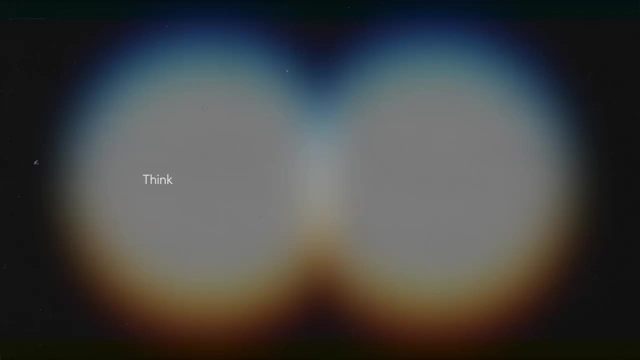 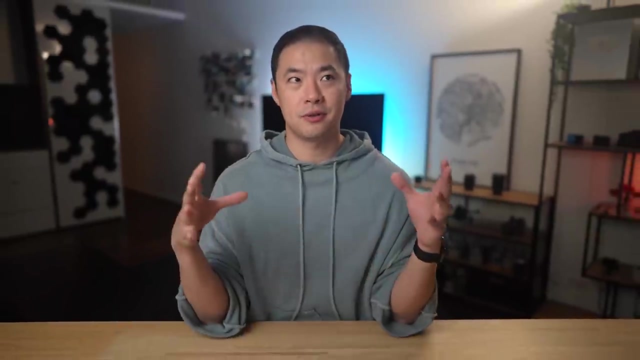 means that you may get an unintentionally blurry image and you can never unblur a blurry shot. You can remove noise from a noisy shot and, because of this, think of ISO last when it comes to setting up your shots. and that leads me to bringing all of this together. So when I'm approaching a 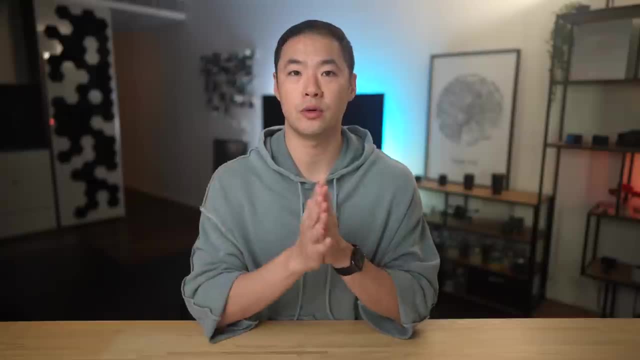 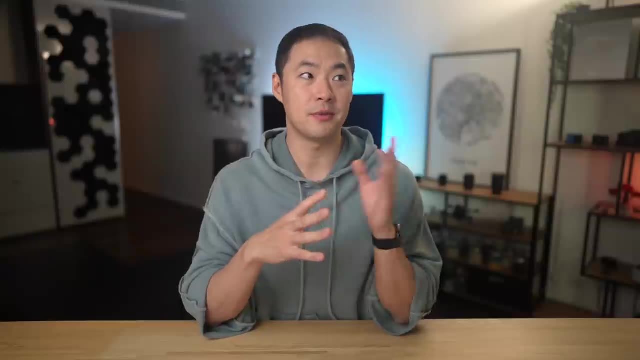 scene I want to take a photo of. I'll always think about doing it in this order. First, I will think about whether or not I want my subject in my image to be blurry or be frozen. 99% of the time it's going to be frozen. so that's my decision, made for me, and I'll adjust my shutter speed according to. 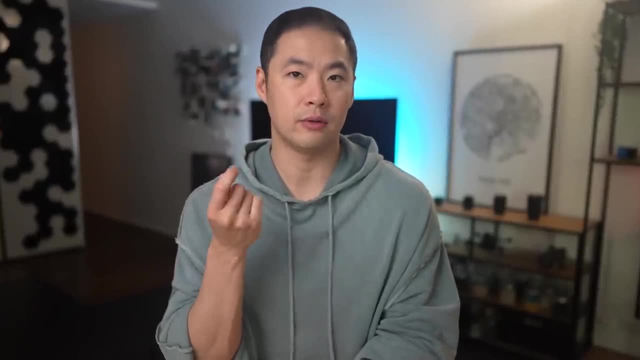 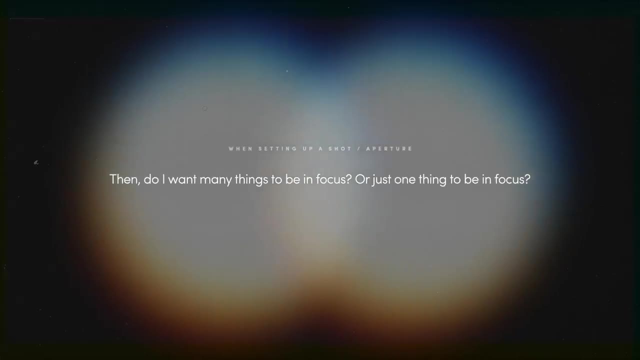 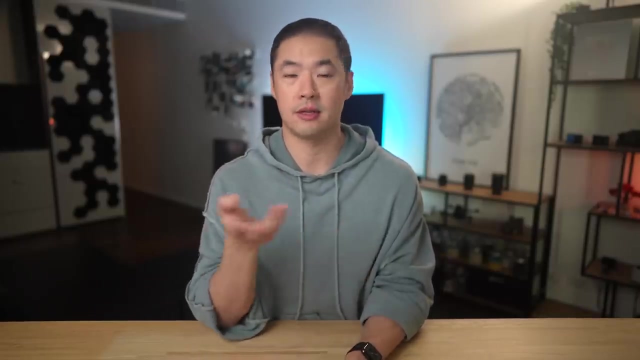 what I want to see, and usually I will go a little bit faster than I think I'll need just to be on the safe side. Then I'll think about depth of field. Do I want many things to be in focus or do I just want one thing to be in focus? and usually this change will happen depending on what I'm shooting. 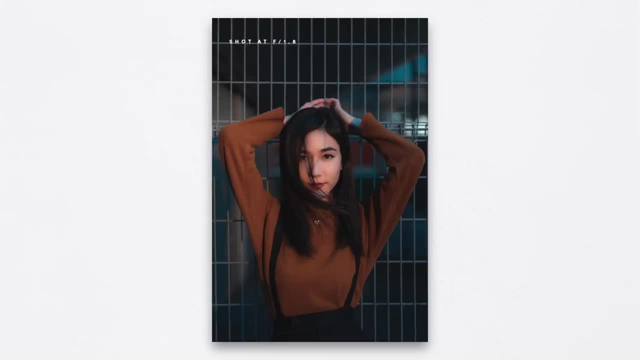 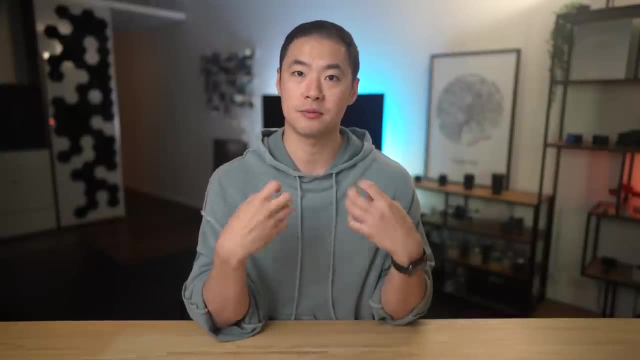 like whether or not it's a landscape or it's a portrait, or if I have a subject in the foreground, and so on. Most of the time, I actually shoot as large as I can get in terms of aperture, because I like to have as much light gathering as possible. 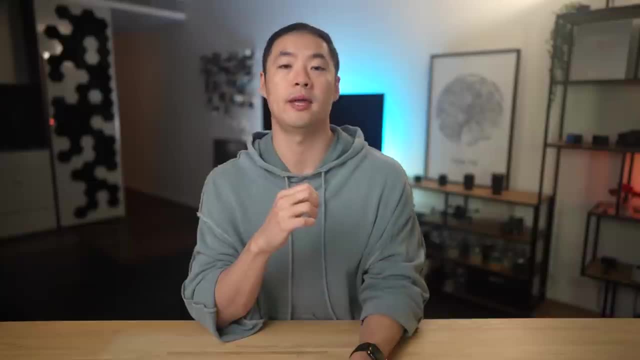 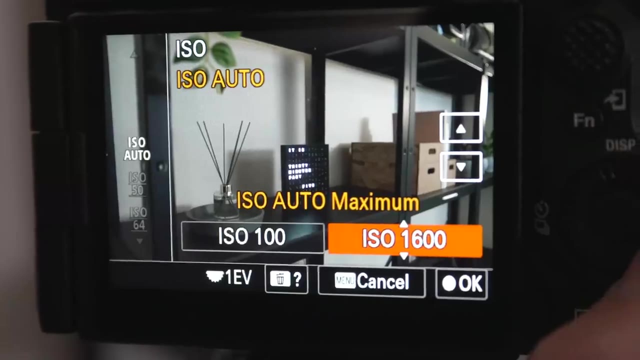 Prime lenses for portraits, or I'm shooting things very far away with landscapes. And then, lastly, I'll look at the image and I'll adjust the ISO accordingly. A tip here, if your camera has it, is to use the auto ISO function and have your ISO set in a bracket so that you don't even need to think. 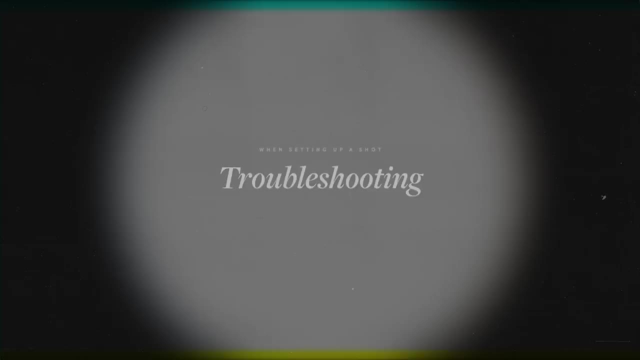 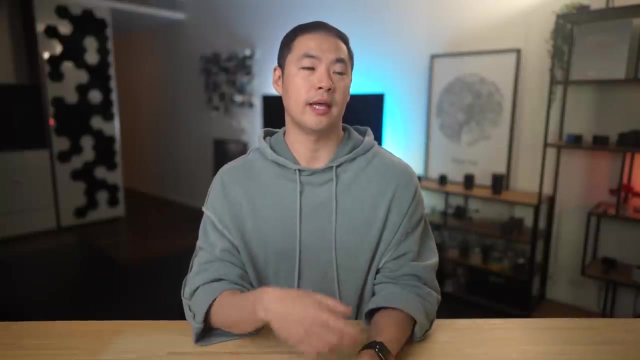 about it and you can let your camera handle it all. Now what do you do if the image is either too bright or too dark? Now, if the image is too dark, you need more light. so usually I will have my shutter speed and aperture dialed in to the image and I'll adjust the ISO accordingly.